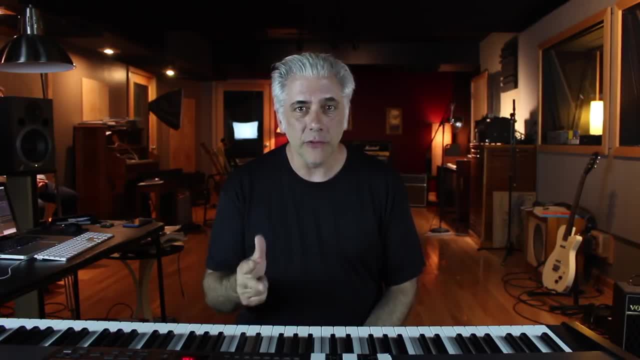 Here's pattern: three, One, two, three, four, One and a two and a Three and a three and a four and a. Here's pattern: four, One, two, three, four, One E and a, two, E and a, three, E and a four, E and a. 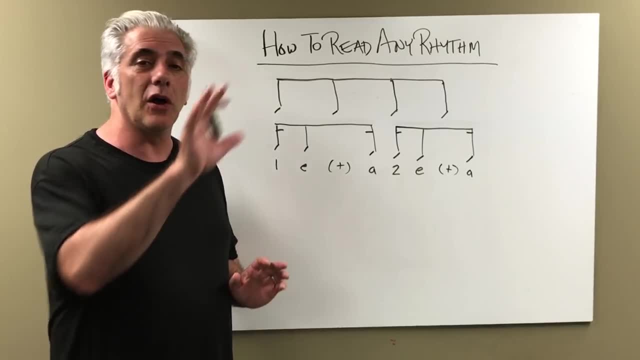 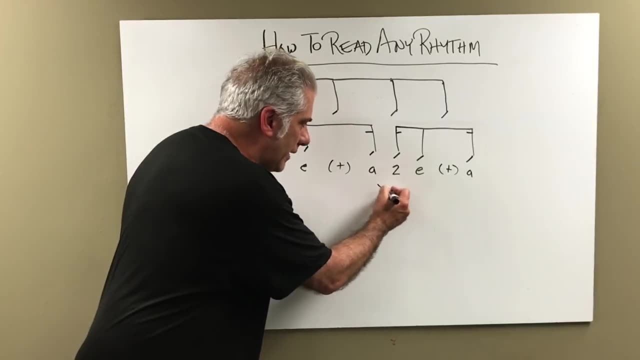 Anytime you have a fourth 16th note in a grouping, it always belongs to the next set of 16ths. Okay, So it'd be one E and a two a two. So you want to make these. This is going to belong to the next one. 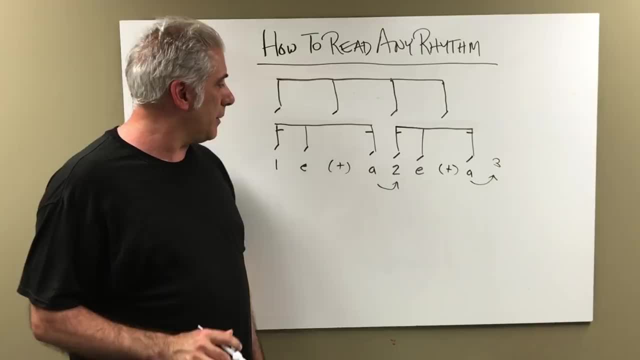 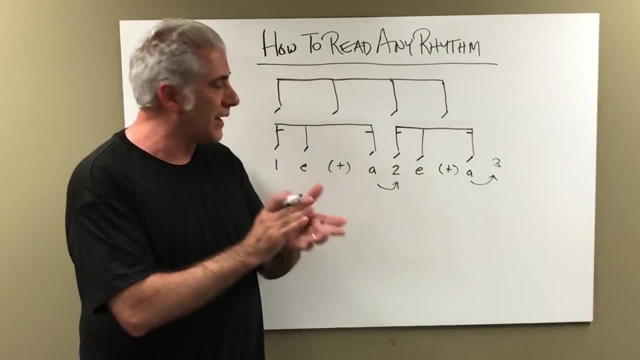 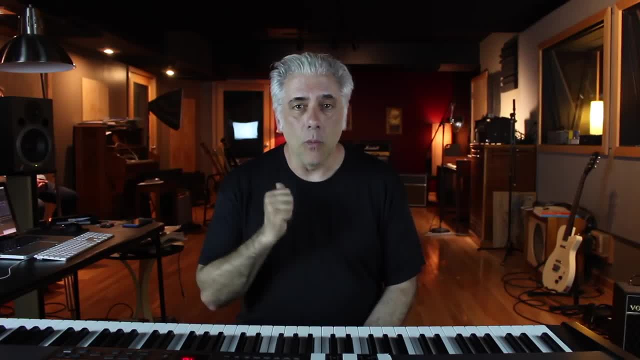 So it's a pickup to the next grouping. Here's pattern five: One, two, three, four. One a, two a, three a, four, a. And the last pattern, number six, goes like this: One, two, three, four. 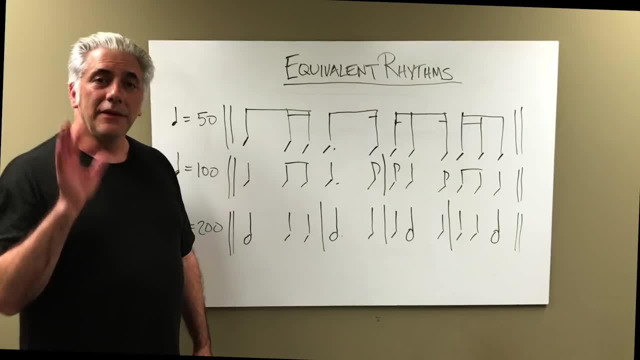 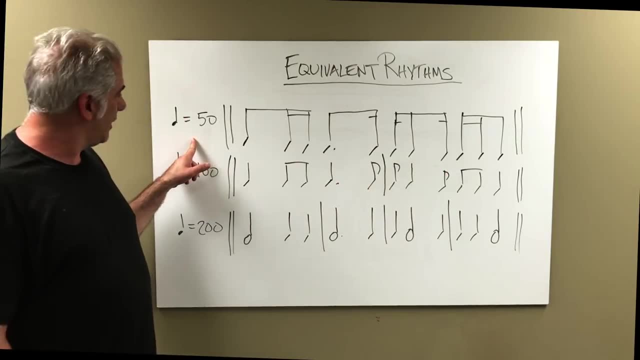 One, two, three, four. Next, I'd like to talk about equivalent rhythms. All of these rhythms Sound the same If you look at the BPMs. this rhythm at 50 BPMs sounds identical to this rhythm at a hundred BPMs. 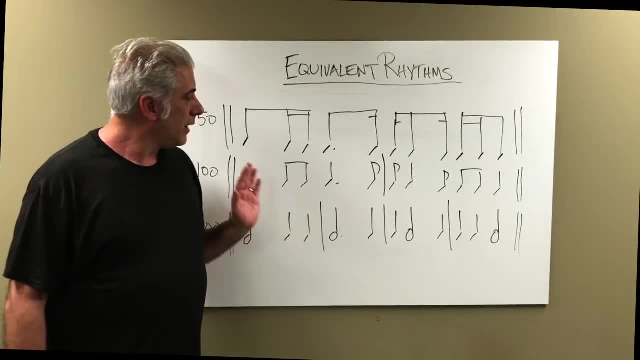 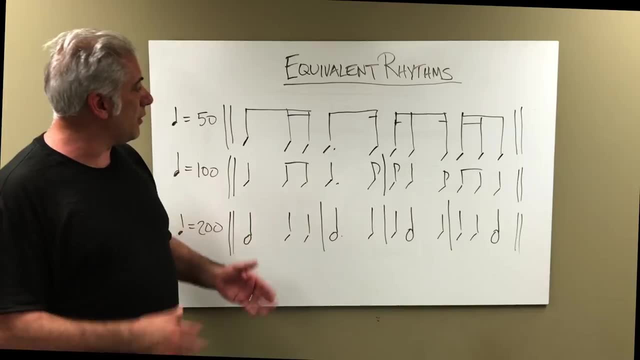 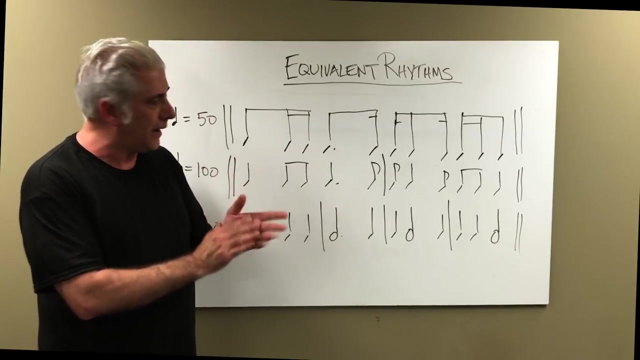 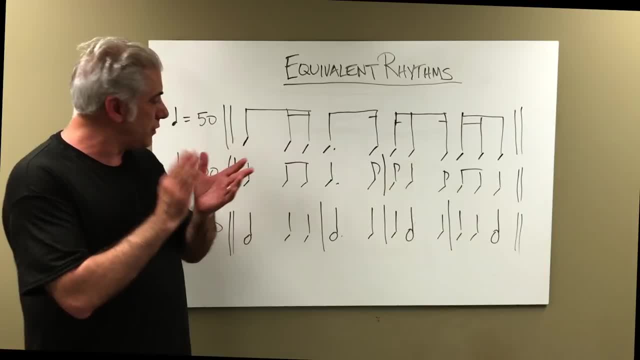 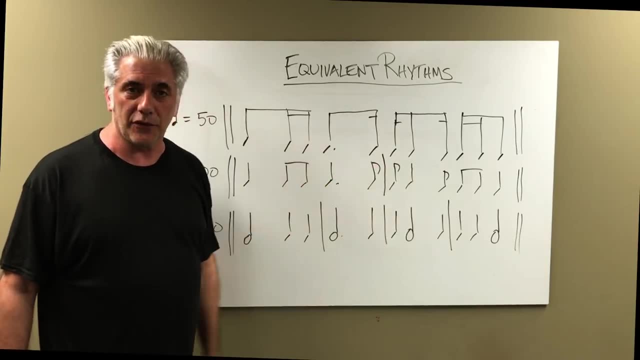 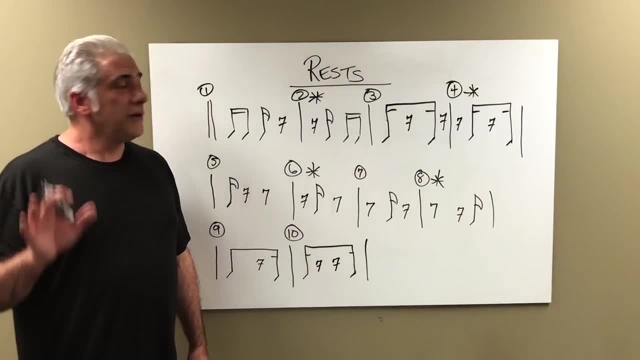 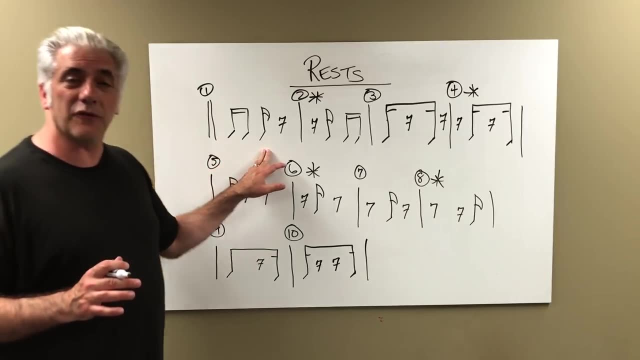 Okay, So let's talk about rests next. Now with rest, many of these patterns sound identical to the other ones, Just the 16th note is shorter. For example, this pattern, this first pattern: Da da, da, da, da, da da. 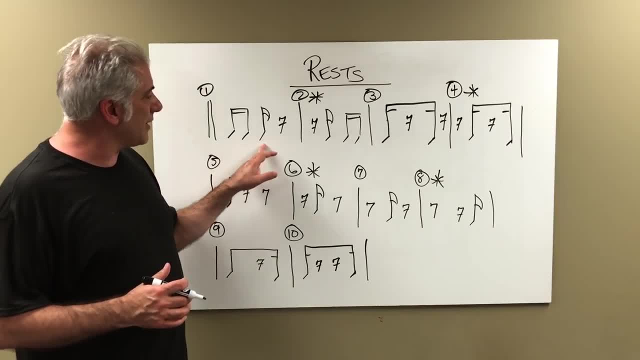 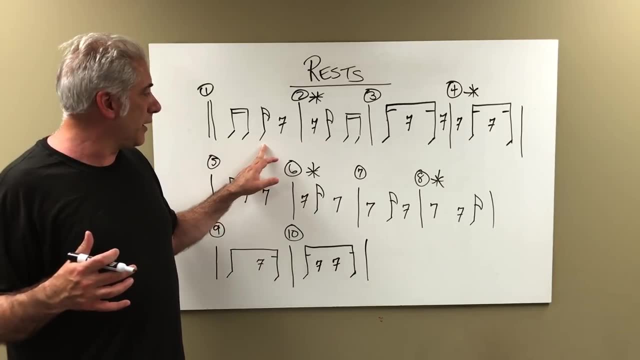 One e and One e and Okay, It sounds like this. It would be a short eighth note which you could write it either way, And you'll see rhythms written this way many, many times where you can have an eighth note with a dot on it. 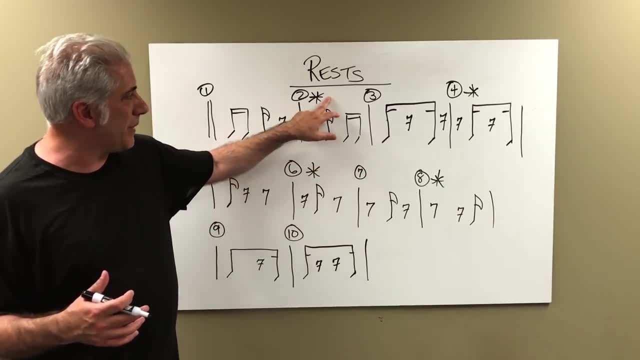 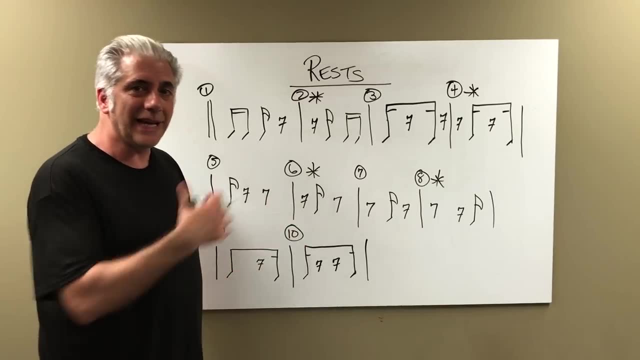 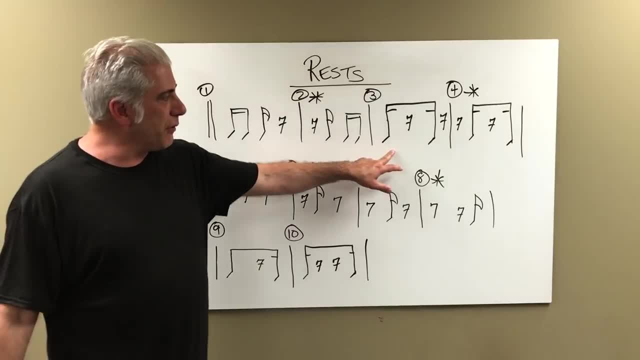 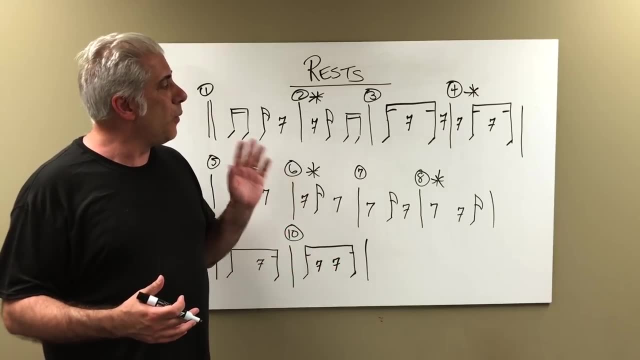 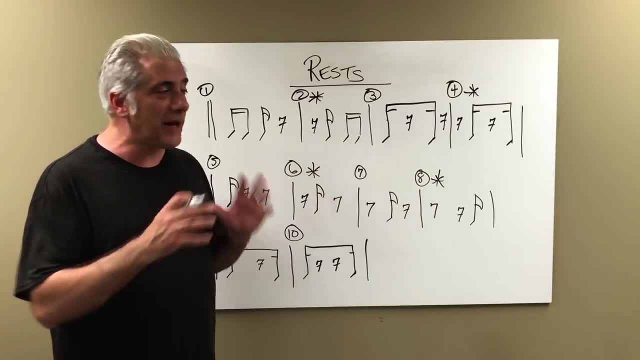 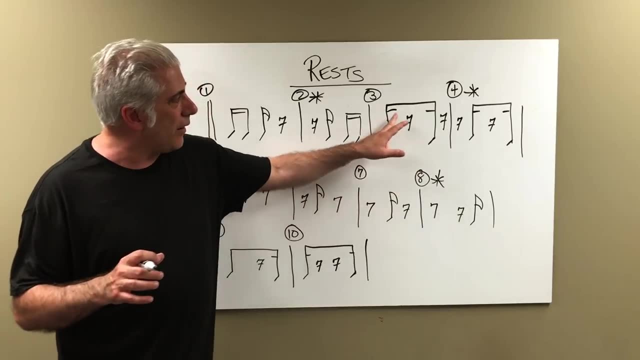 So that that, that that They're just short. So if you wanted somebody to play articulate short, if you're playing a trumpet part, for example, this rhythm you would see played commonly. Now I wrote it this way, with a beam, because it's more of a modern way to write it. 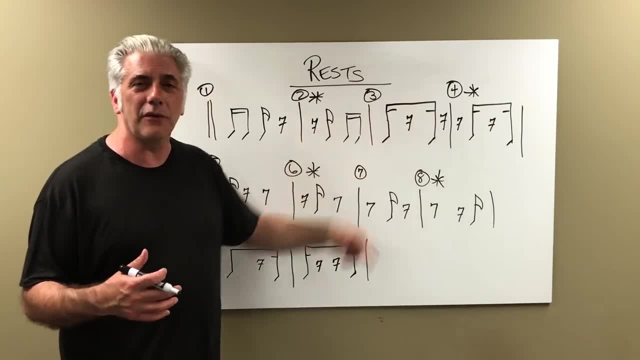 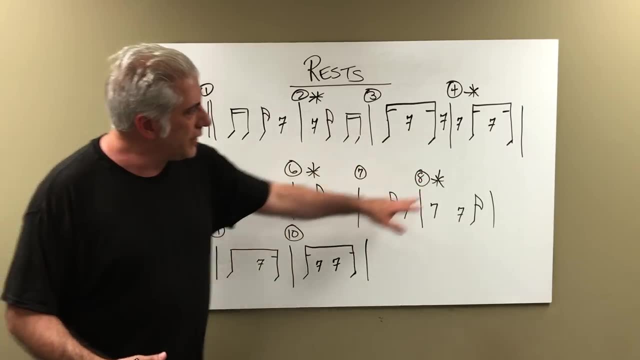 Instead of writing: a 16th note, 16th rest, another 16th note, another 16th note to rest rest. Typically, you would see that in orchestral writing you'll see this as a shortcut. This is a unique rhythm, so it'd be. 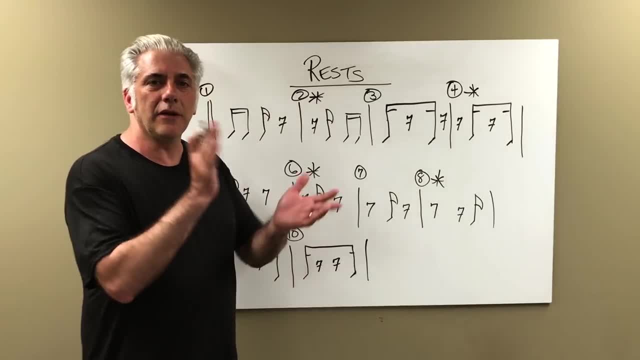 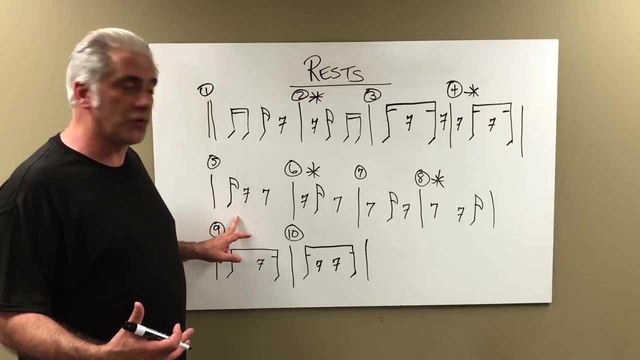 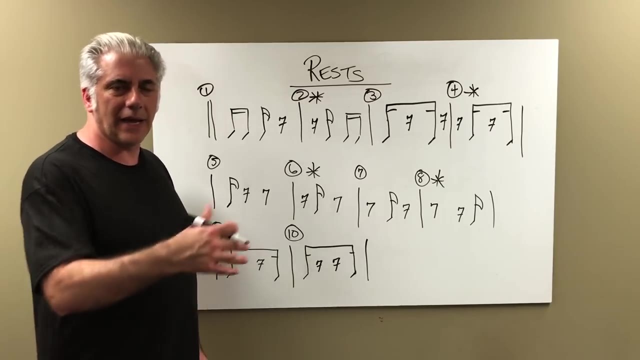 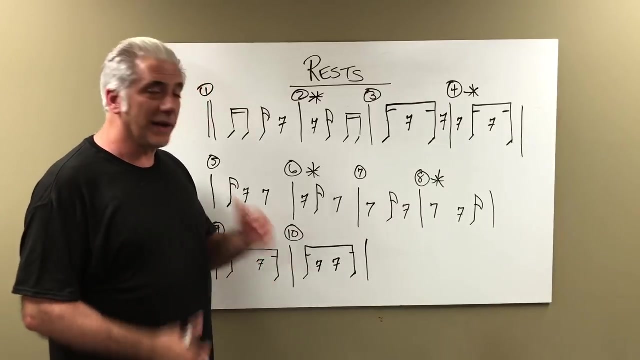 one e and uh one e and uh three, four, ah, ah. number five you could have written as an eighth note with a dot on it. so it's short, but it'd be like one hand, two hand, three hand, so that's not unique. number six here is unique: rest up, rest up. so one e and one e and one e and. 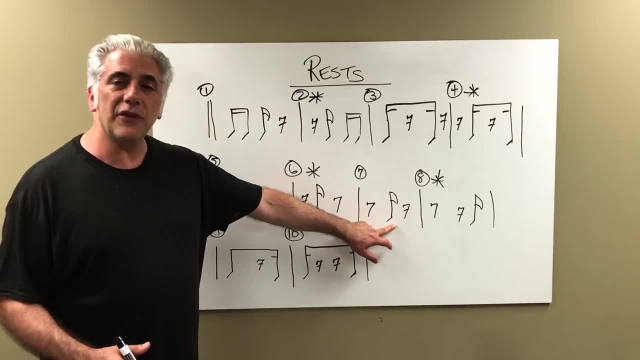 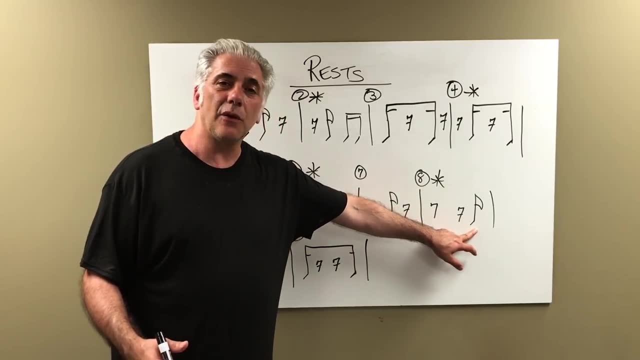 number seven, since the sixteenth note lies on a beat. it's not unique because it comes on. and number eight is a unique rhythm because we have a sixteenth note on the last. so it would be one e and ah, three, four, one e and oh, one e and oh one. 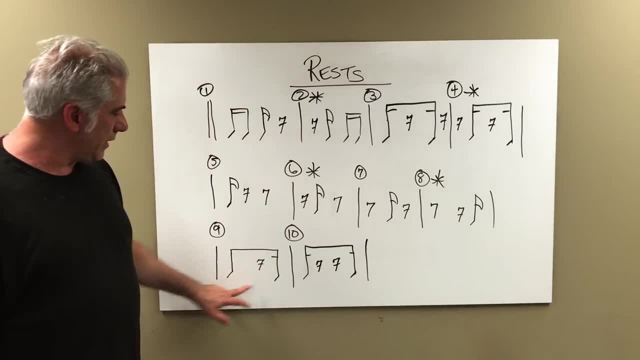 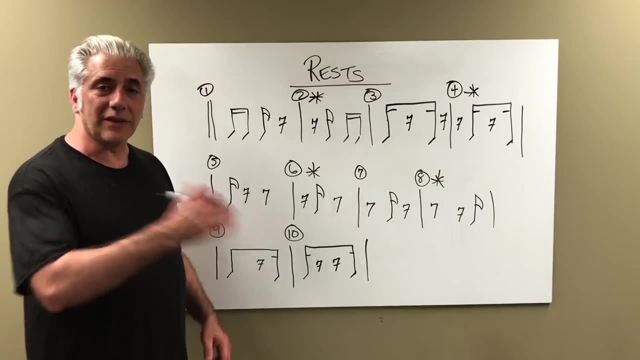 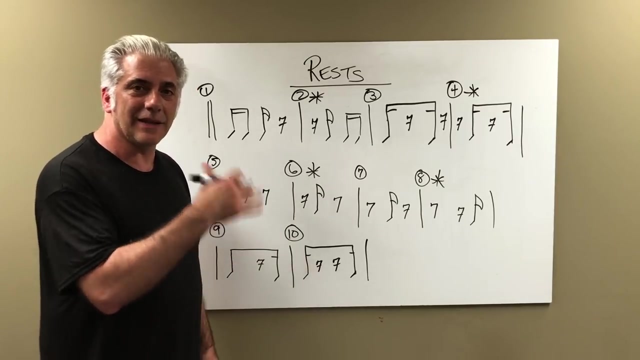 e and uh one e and uh, okay, number nine and number ten sound identical. actually, if you went now, this is a an eighth note, rest sixteenth note, and this is sixteenth rest, rest sixteenth. but you could say it's da da, da, da da da. this would be da da da, this would be that, that, that, that, that, that. 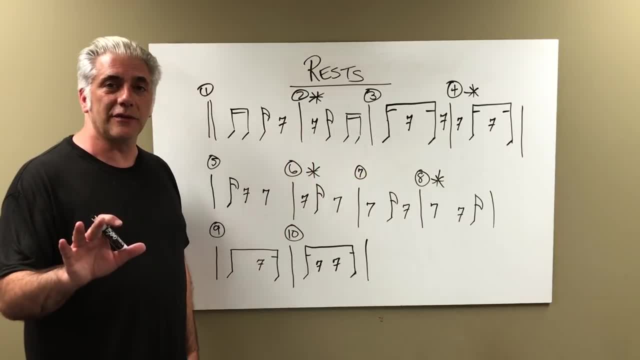 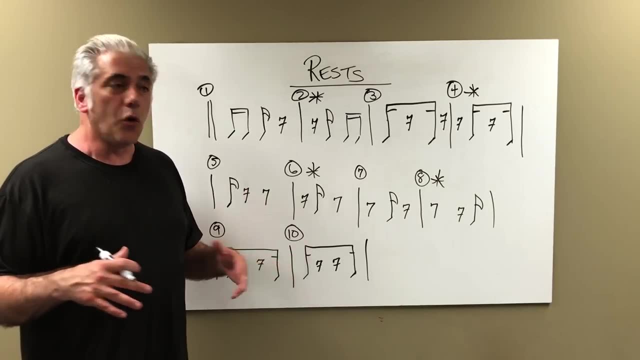 all you need to do is memorize these ten patterns with the rests, combine them with the six patterns from before and you have all the possible combinations of four sixteenth notes, or if you make them eighth notes, it's the same thing. change everything here to eighth notes and 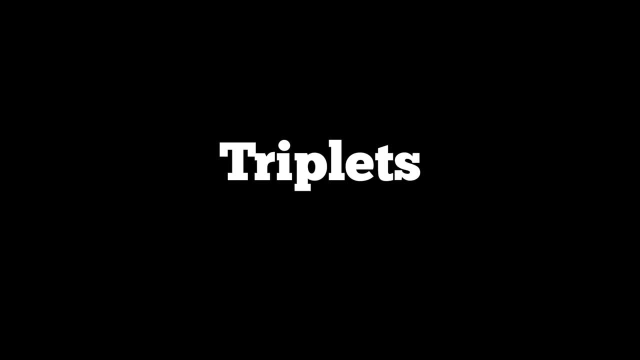 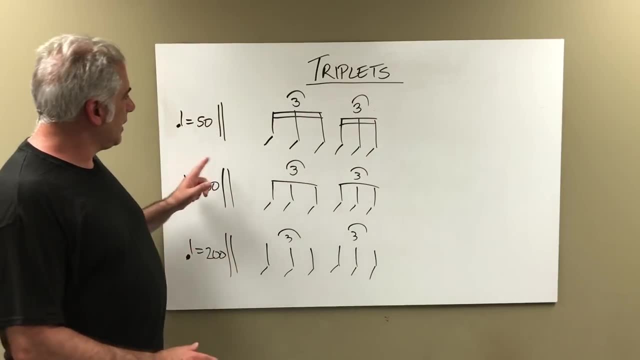 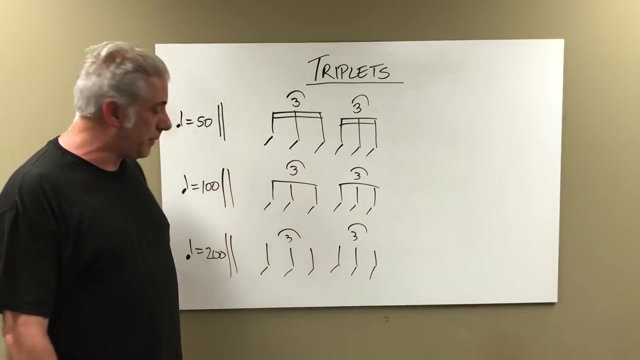 then you know how to perform these same rhythms as eighth notes. okay, the last thing we're going to talk about are triplets. now i did the same thing with these triplet equivalents. triplet sixteenth notes at 50 bpms are going to sound the same as eighth note. triplets at 100 bpm, which are: 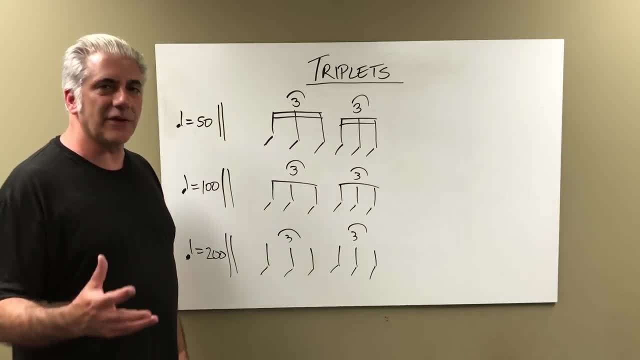 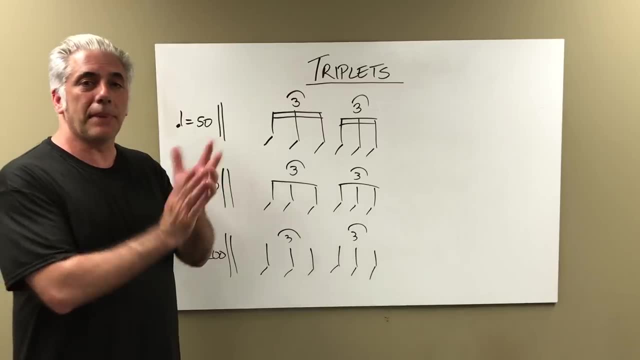 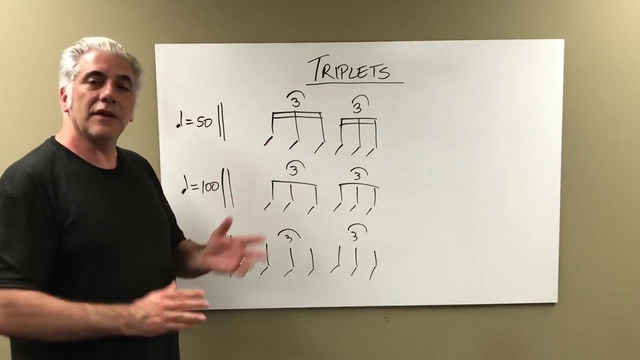 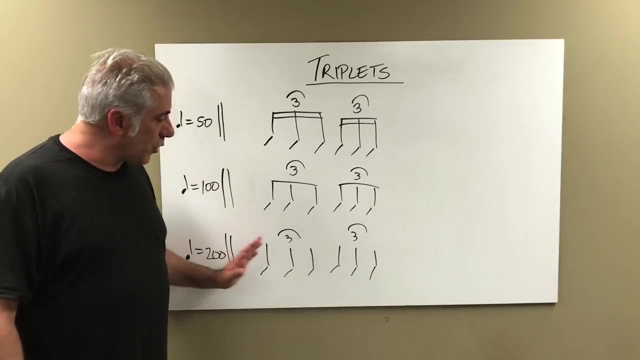 the same as quarter note triplets at 200 bpms, but in reality the way that these would work is this: if we put these all against a quarter note, the triplet sixteenth would sound like this: the eighth note triplet would sound like this: three, four, with the down beats on both of those falling on strong beats, but with the quarter note triplets. 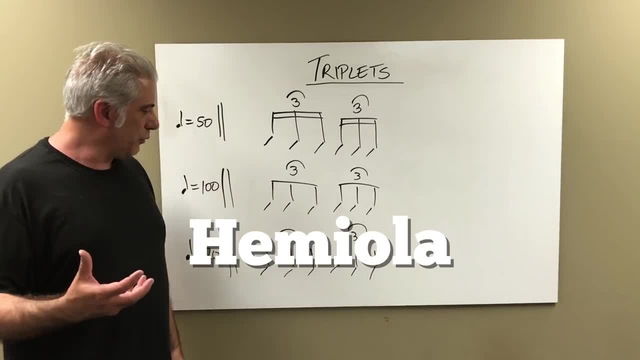 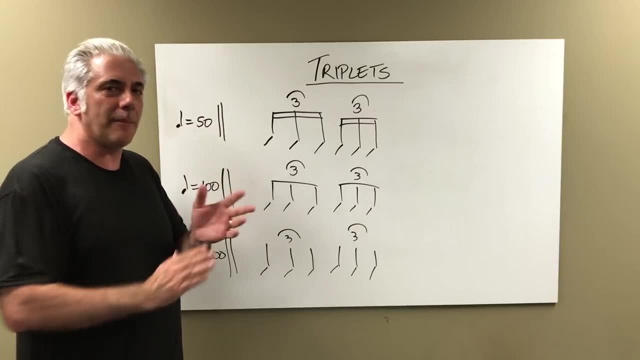 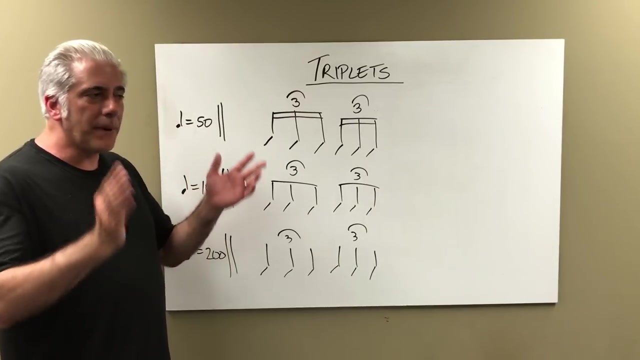 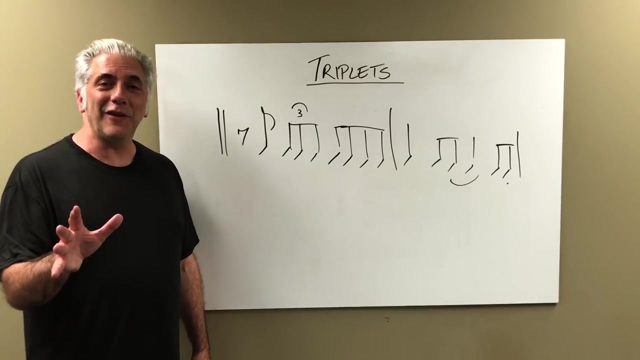 it's a little bit different. you get this three against two feel, or hemiola, which would be this pattern, like this: three, four. so every half note you fall on a downbeat: three, four. that's a three against two pattern or a hemiola. any of you that watch any of my jazz videos will. 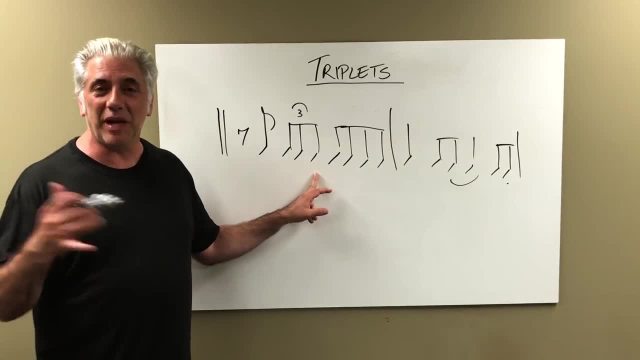 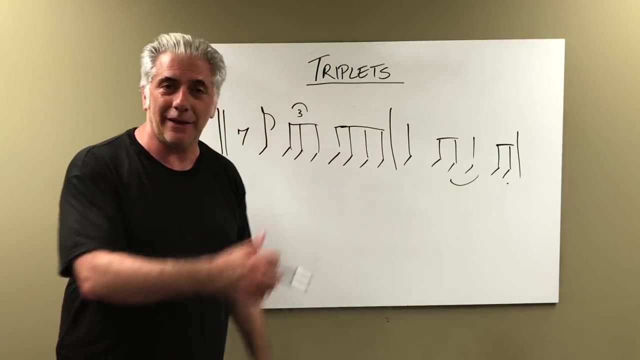 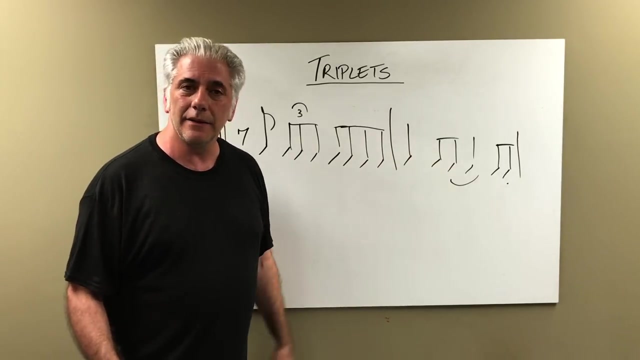 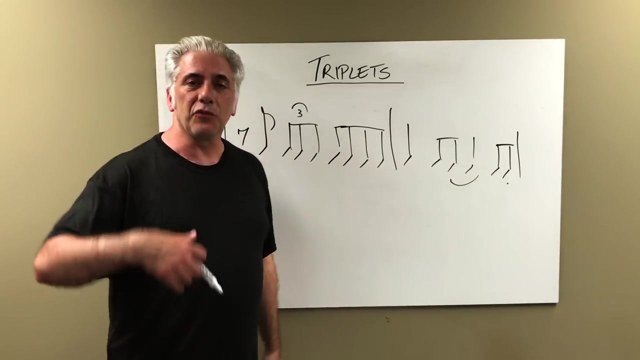 know that we use triplets a lot on the second beat in bebop because that's kind of a charlie parker thing or really a bebop thing. raspid okay. now this is a tied note but really it's playing okay. in jazz we play swing eighth notes. see these struggling, played as triplets. 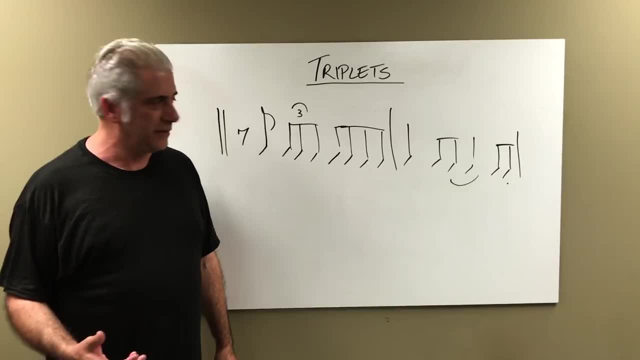 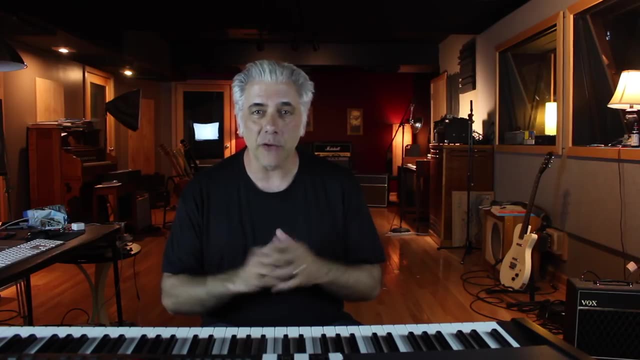 with a triplet field. it's called the swing field. these are called swing eighths. so three, four sound Okay. let's take a look at a real-world example. This is John Williams' Superman theme. Let's take a look at this rhythm. 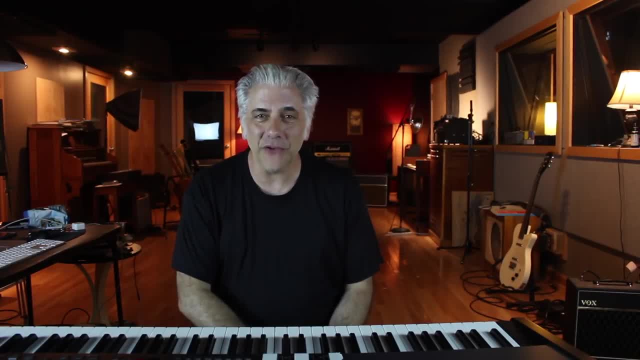 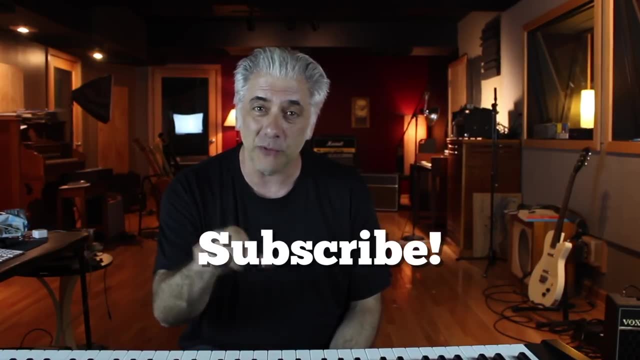 That's all for now. Please subscribe here to my Everything Music YouTube channel and if you're interested in the Beato book, you can write me at rickbeato1 at gmailcom. Don't forget to hit the subscribe button and the notification button. Thanks for watching. I'm Rick Beato.